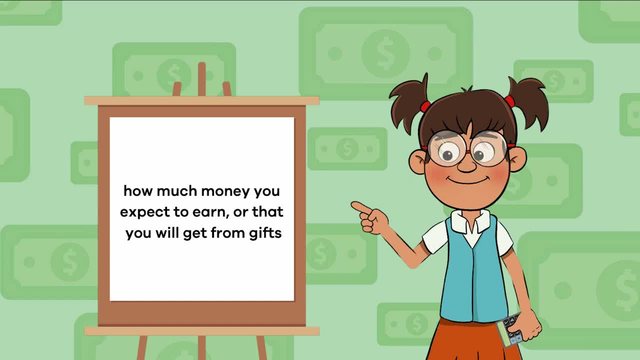 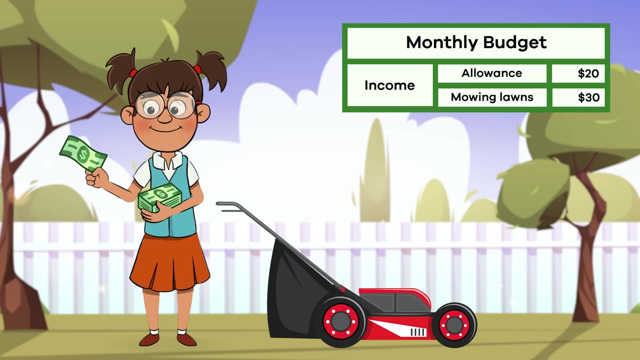 First you need to figure out how much money you expect to earn Or that you will get from gifts. That is called your income. Each month, Frankie gets a $20 allowance: $30 for mowing lawns and $20 for pet sitting. 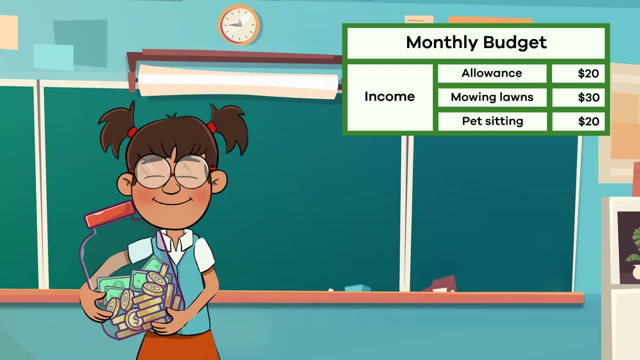 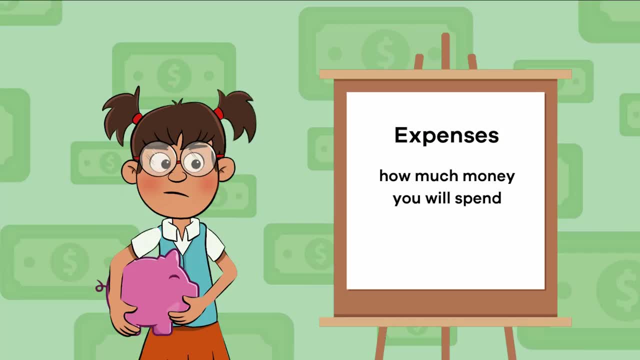 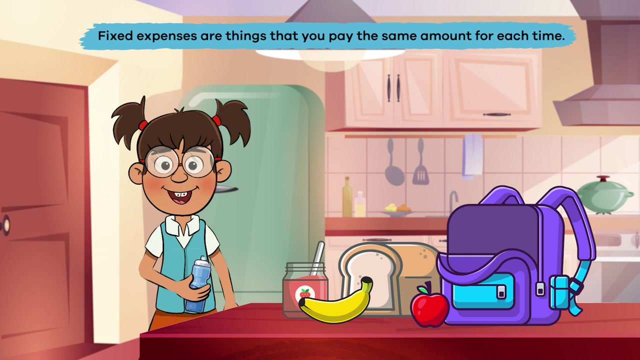 which means she will have a monthly income of $70.. Next Frankie has to figure out how much money she thinks she will spend. There are two types of expenses – fixed and variable. Fixed expenses are things you pay the same amount for each time, like school lunch. 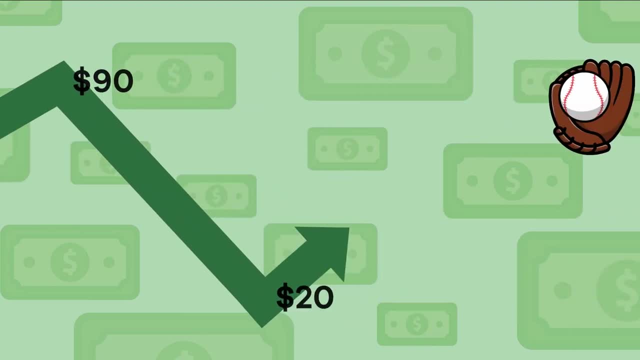 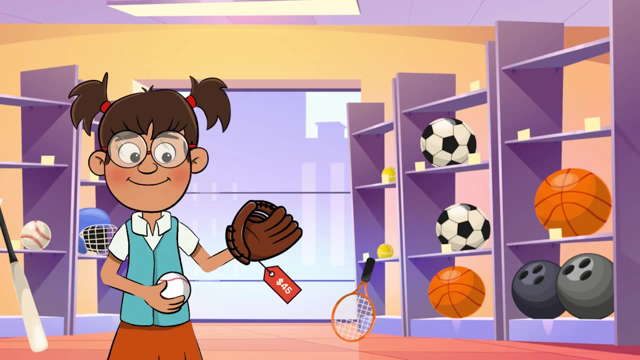 Variable expenses are the opposite. They vary or change. For instance, one month Frankie wants to buy a pair of pants and the next time she wants to buy an extra pair of gloves. The prices of these items vary greatly between school lunches and expenses. 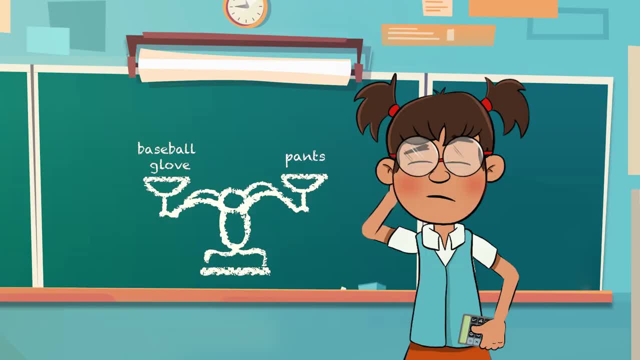 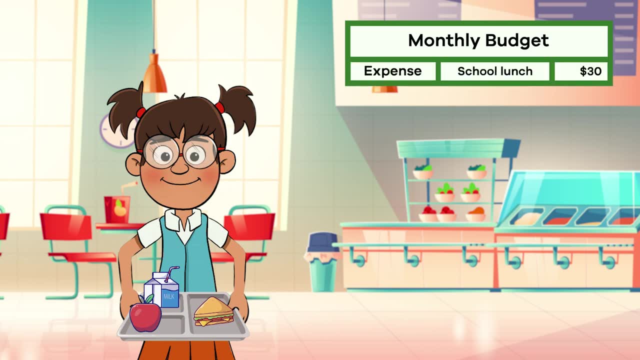 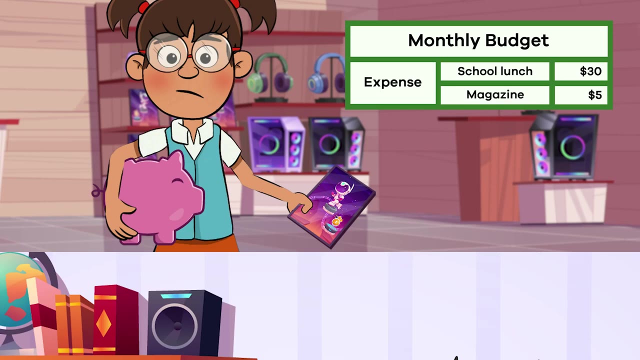 are different from each other, which means that the expenses are harder to plan for. This month, Frankie will spend $30 on school lunch and she wants to spend $5 on a monthly online magazine subscription, but she also wants to buy a video game that costs $20.. 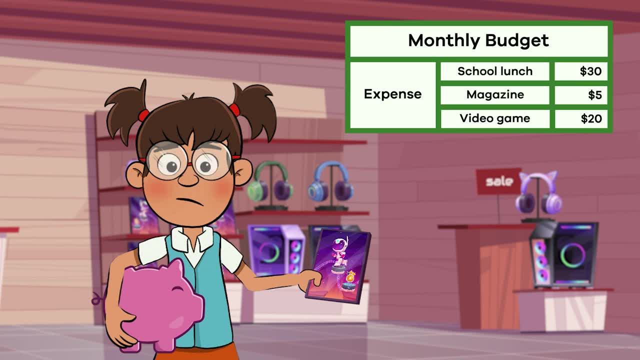 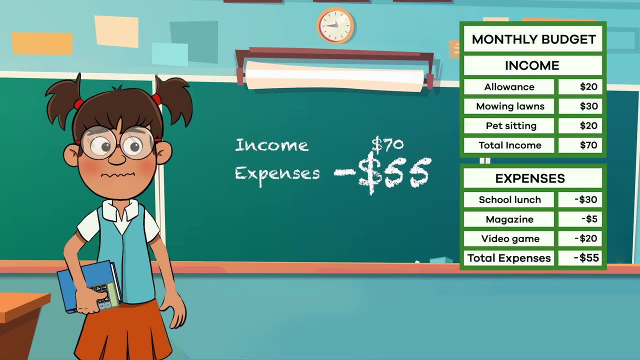 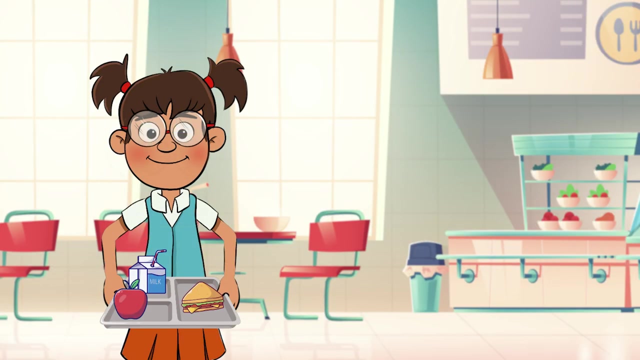 Will she have enough for the video game? Let's look at her budget and see. If we compare Frankie's income with her expenses, we see that she does in fact have enough money to buy the video game with $15 to spare. It is awesome that Frankie has enough money to pay for her needs and her wants. 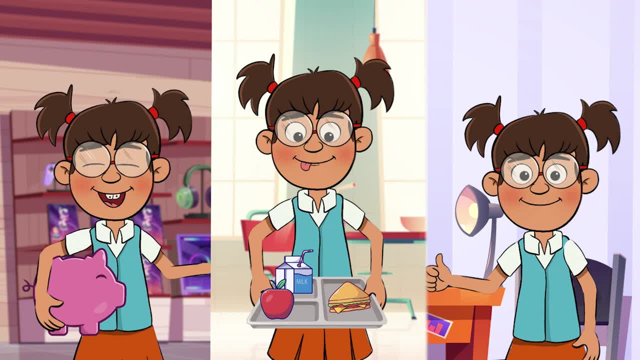 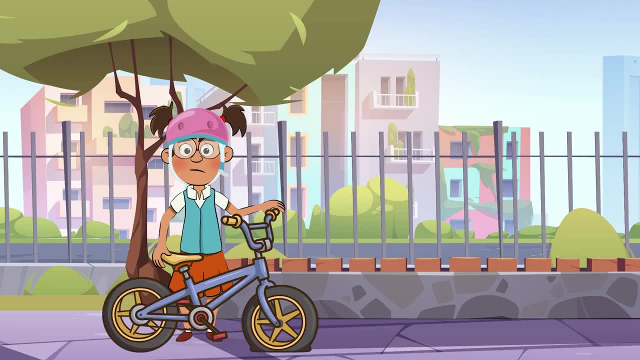 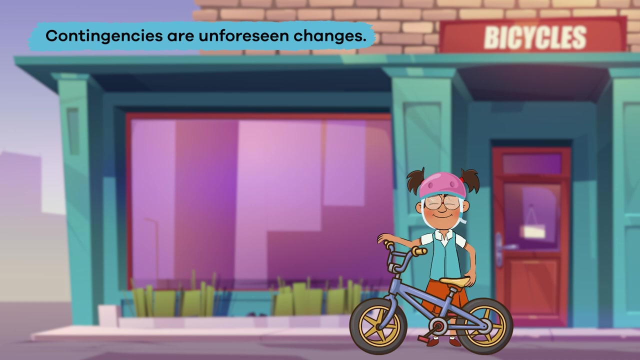 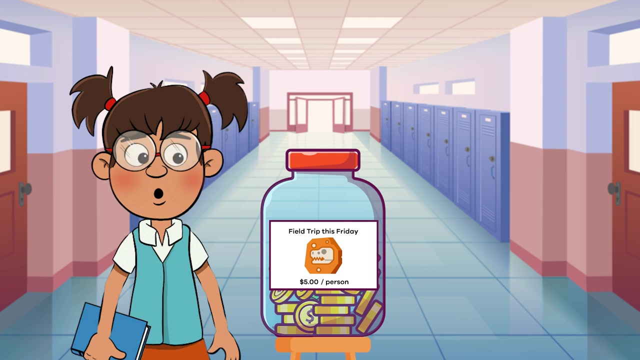 But it is important to remember that income and expenses are often estimated. Sometimes unexpected expenses happen, so you have to make sure your budget is flexible and that you save for contingencies which are unforeseen changes. Frankie finds out that she has to contribute $5 to her school if she wants to go on a field. 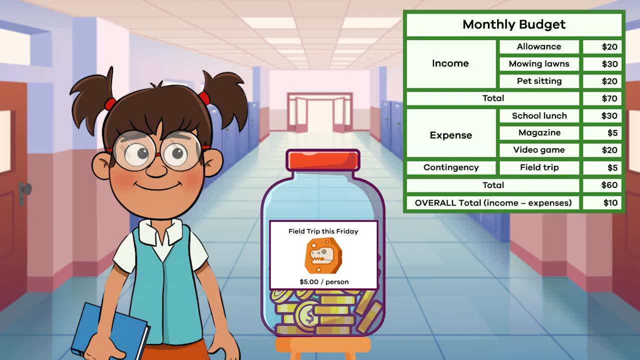 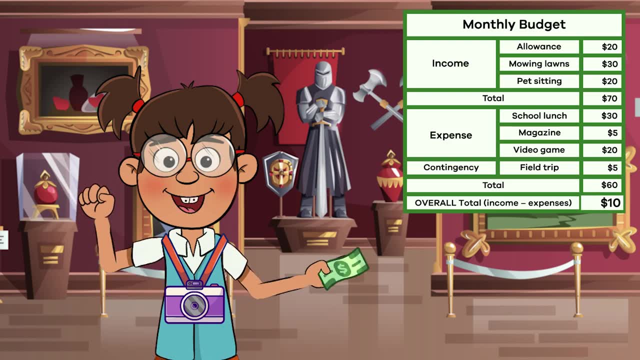 trip to the museum. Luckily, this contingency did not happen. This means that Frankie will have to spend $20 on a monthly online magazine subscription. it doesn't make much sense with her savings account, But she can afford it with $10, it's definitely worth her saving. 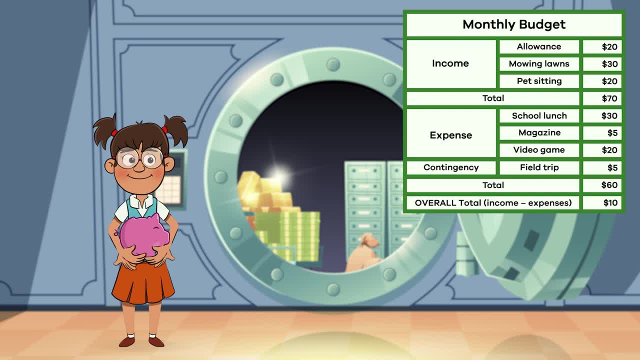 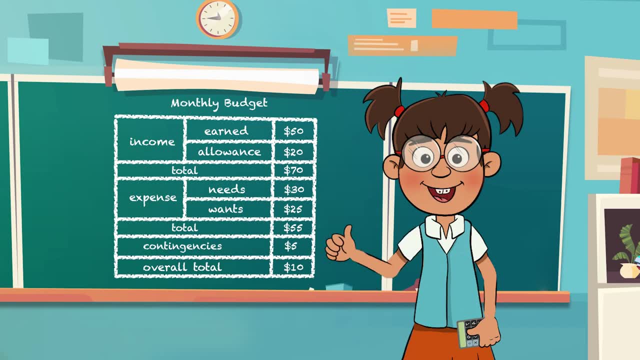 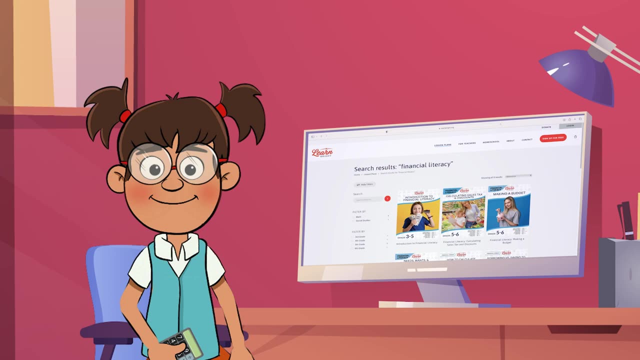 Now, that is some effective budgeting. Now it is your turn At home. try this exercise out for yourself. You can download this lesson plan on LearnBrightorg and print off some of these information, But don't forget to share this video in your native language with your friends and family. 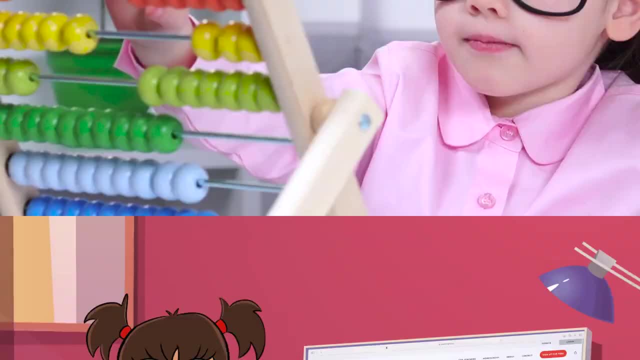 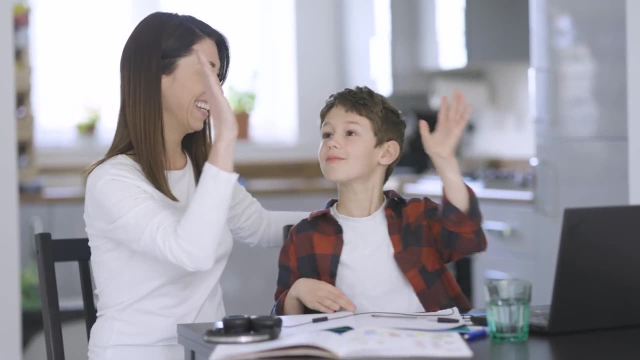 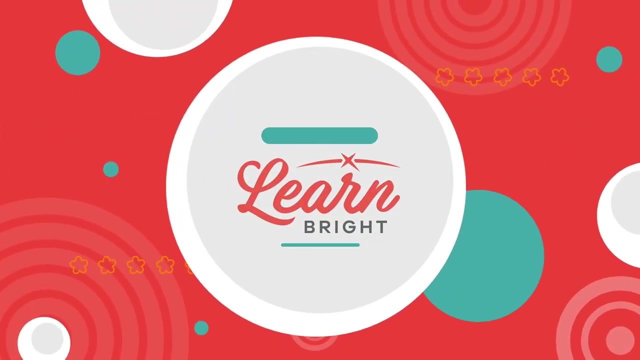 And don't forget to subscribe to our channel for more videos like this. Thank you off some practice pages. Before you know it, you will be a budgeting pro and on your way to becoming financially literate. Hope you had fun learning with us. Visit us at learnbrightorg. 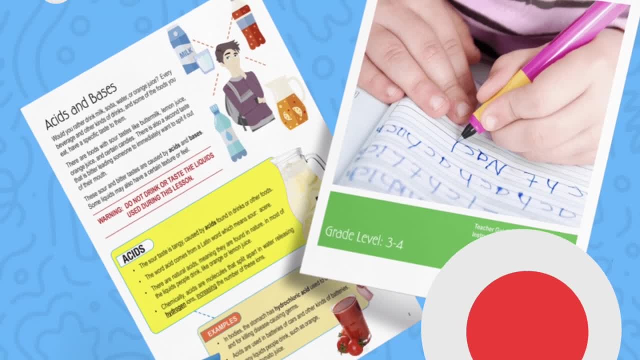 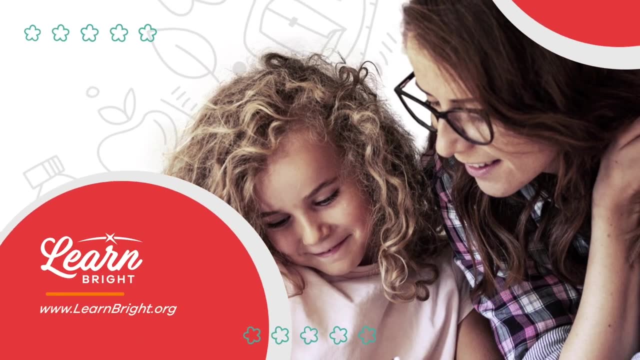 for thousands of free resources and turnkey solutions for teachers and homeschoolers. Thank you, 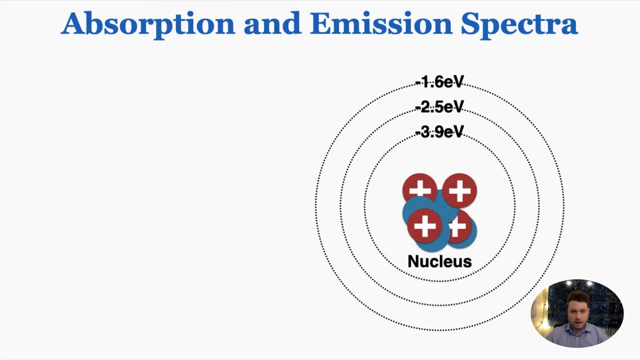 This lecture is going to be about absorption and emission spectra. I'm assuming in this lecture that you've seen the previous lecture on electron energy levels and if you haven't, I've left a link to that in the video description. You'll remember from that lecture that electrons exist at specific 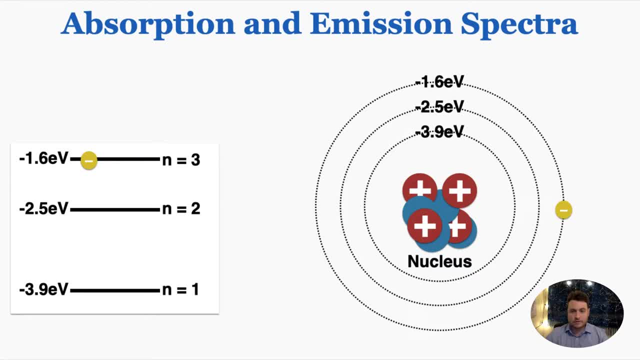 energy levels in atoms, and every single time an electron goes down an energy level it emits a photon of that exact same amount of energy. So just observing this electron here, I can see that every time it drops a certain amount of energy in electron volts it emits a photon of the same 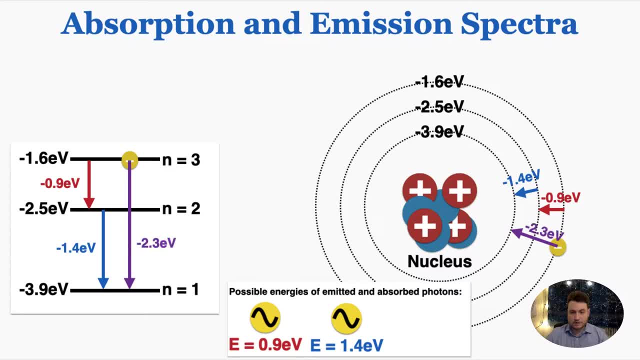 energy. and if we want to increase an electron's energy in an atom, we have to add a photon to it, where the photon is absorbed by the atom, and the photon has to have that exact amount of energy required to get the electron to the correct energy level, because electrons cannot exist between 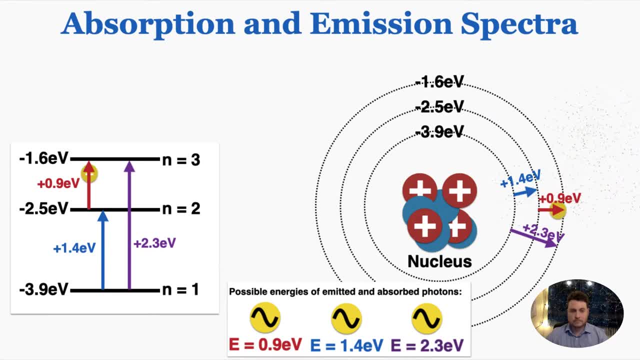 energy levels. In another lecture on photons, which I've also linked in the description, I talked about how, if we know the energy of a photon, we can also automatically know its wavelength. using this equation. Before I use that, I'm going to show you how to use a photon to know its wavelength.